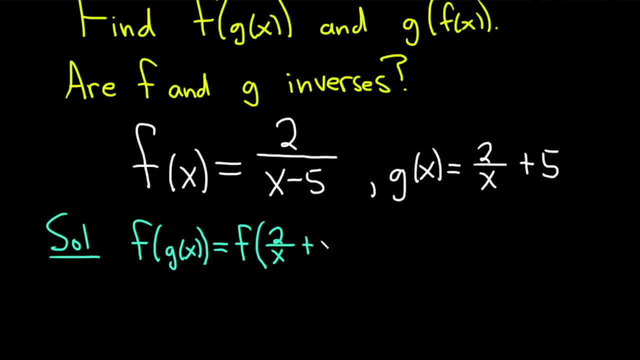 2 over x. Very nice. Now we're going to take this and plug it into f, So this whole thing here is basically our x. Up here we have f of x equals 2 over x minus 5.. So this is going to go where. 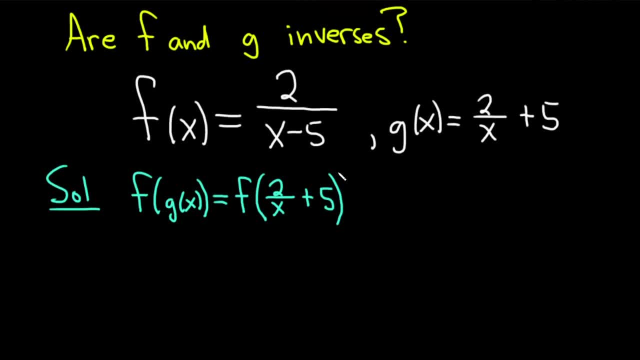 the x is in this function. So now this is equal to 2 over and instead of x. we just have this expression here. So 2 over x minus 5.. 2 over x plus 5.. And then we have the minus and the 5.. So this whole piece here is our. 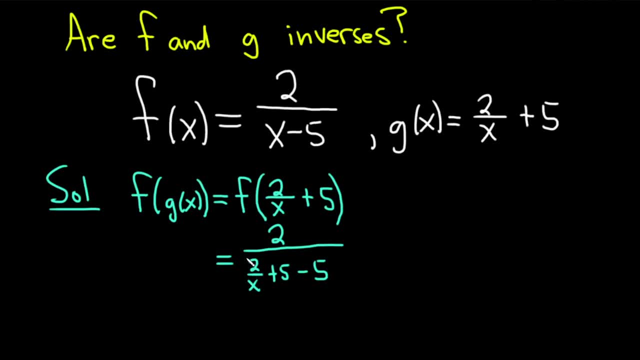 x. Now, because we have a fraction here on the bottom, and to avoid confusion I'm going to put parentheses here. They're already there, but they're implied. There's even parentheses around the 2, except nobody really writes them, because what's the point? But look what happens. 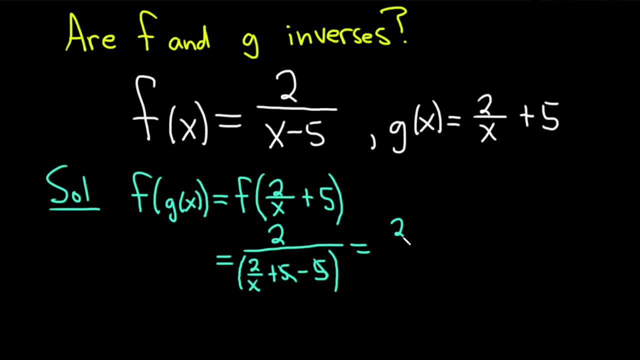 now We get some cancellation and then this is equal to 2 over parentheses, 2 over x. So we have 2 divided by 2 over x. So when you divide you really multiply by the reciprocal, So this is really 2 times and then x over 2.. These cancel and then so you end up with: 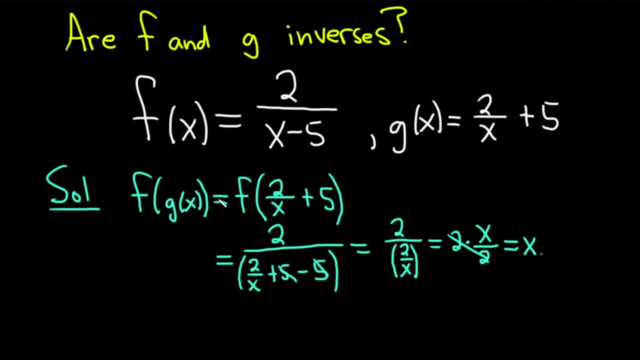 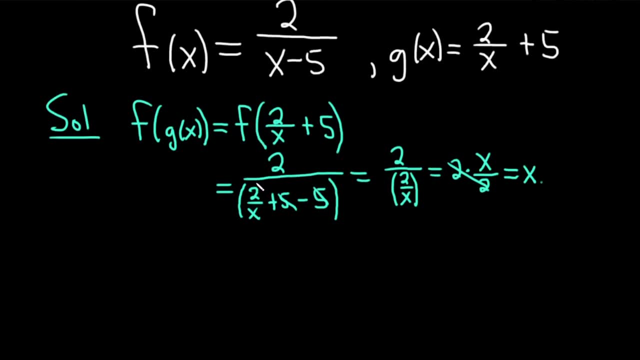 x. That's really really good, because we got x for this one. Now we just have to make sure- or hopefully, we get x when we compute g of f of x, And we will. but let's just go ahead and verify 0.025.. 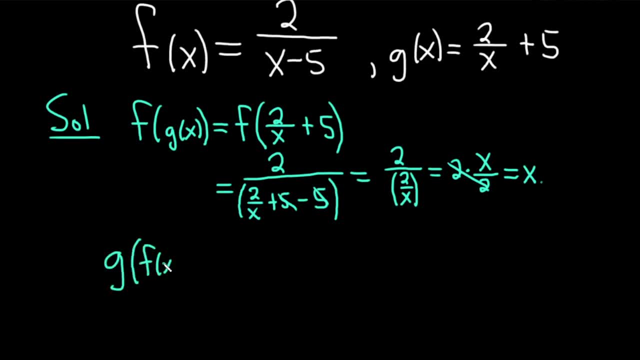 So g of f of x is equal to. so this time we'll start by replacing the inside piece with what it is. This is g of well, f of x is 2 over x minus 5, so this is 2 over x minus 5.. 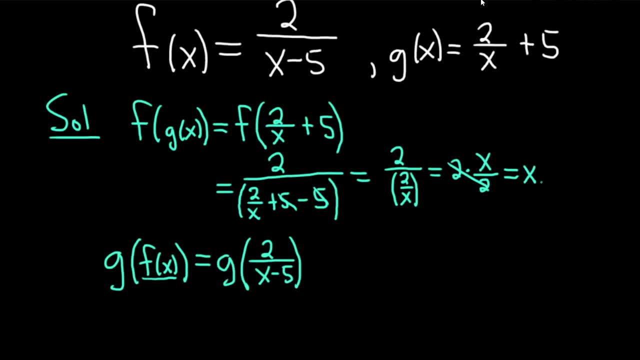 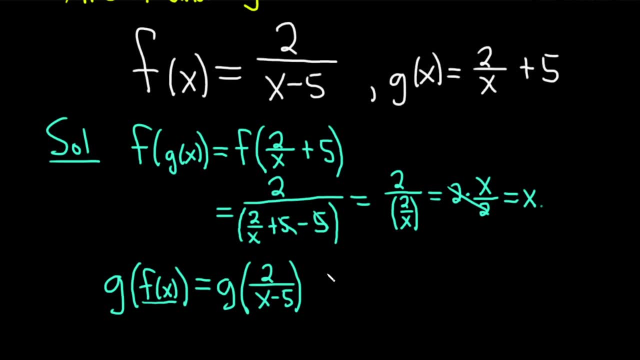 So now we look at g, So g is up here, so it's 2 over x plus 5.. So basically, what we're going to do is put this where the x is in the formula for g, So it's 2 over, and then we have x, but our x is this right.